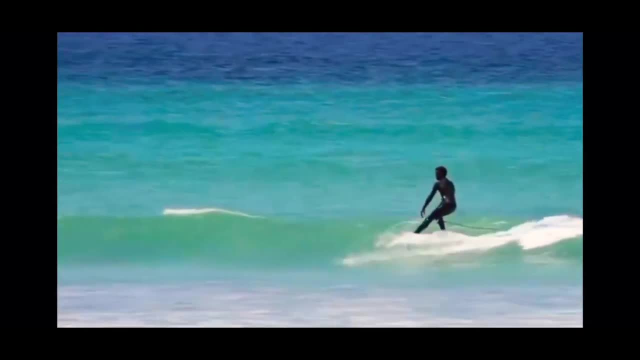 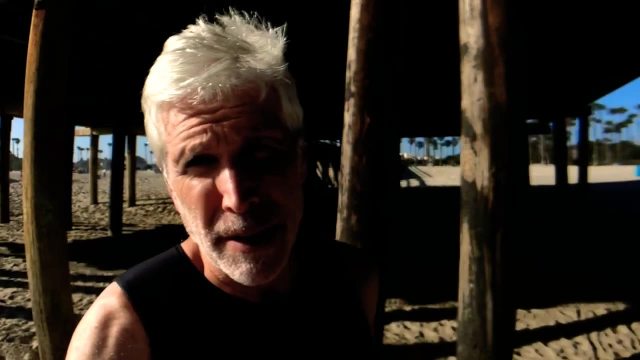 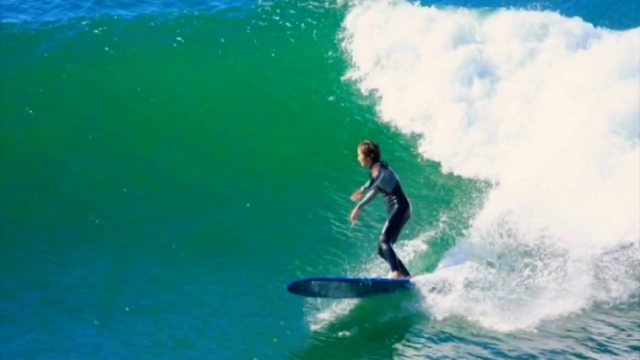 here he said nimble toes Johnson of the SoCal seven developed the hair lip double barrel punching roll right here at Malibu Lagoon or something to that effect. I really didn't know what he was talking about, but it sure was damn important to him. we found our way to the topic of wave. 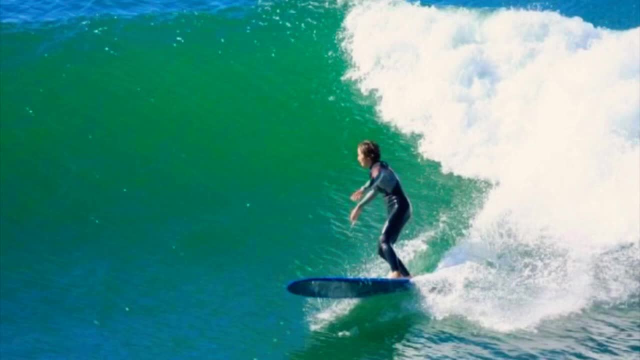 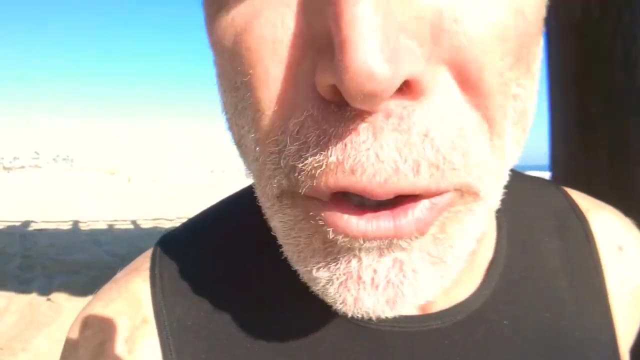 height. when I told him as a proner I look for waves eight to ten feet, it was as if I had just insulted the national flag of surfer douchery. where do you see 10-foot waves in SoCal? how big do you think those waves out there are? I said: 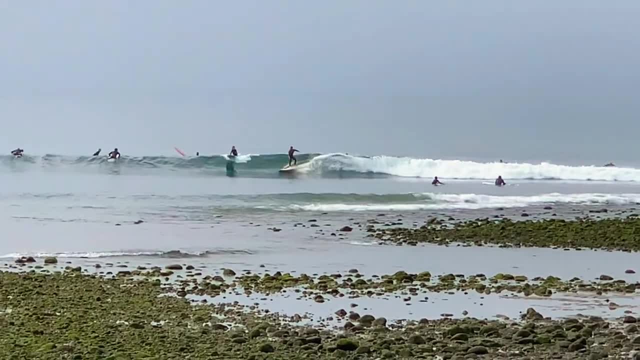 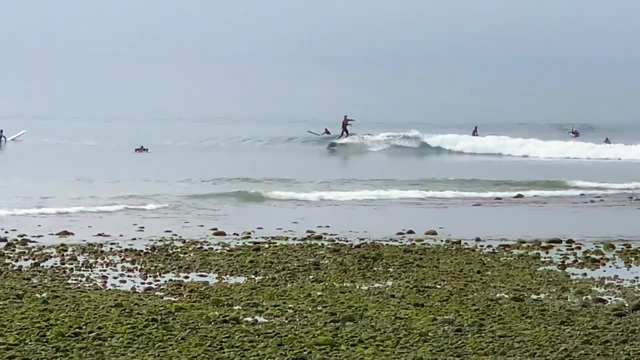 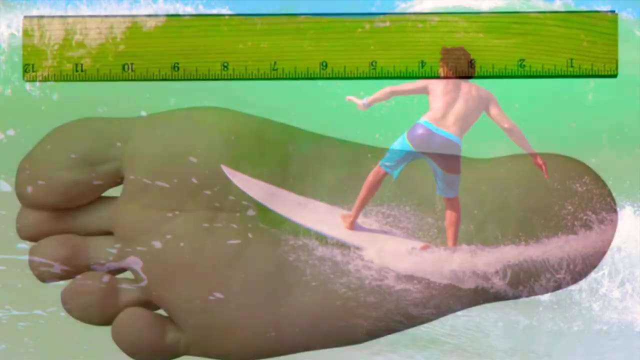 two to three feet. haha, that must be East Coast measuring, you know. he actually said that. then he went on to tell me that the waves I was seeing out there were one foot high and that a wave that reaches the head of a six foot tall person is only three feet. a bit confused on the 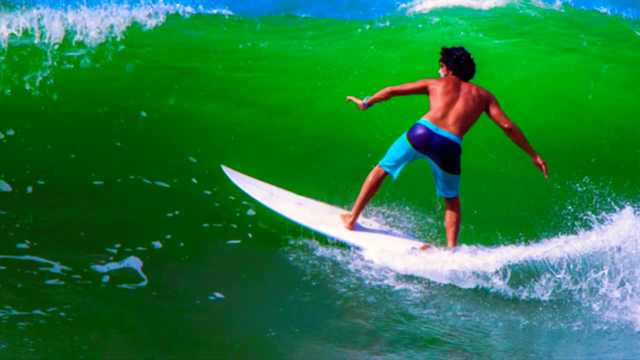 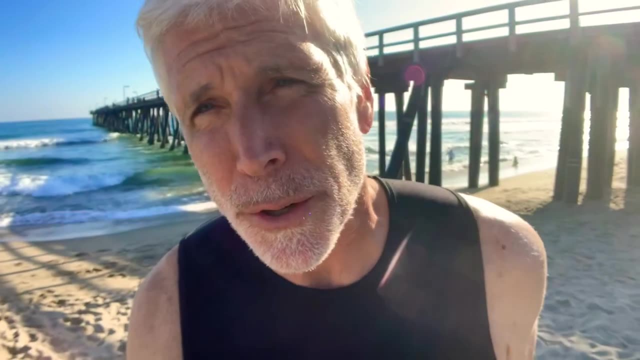 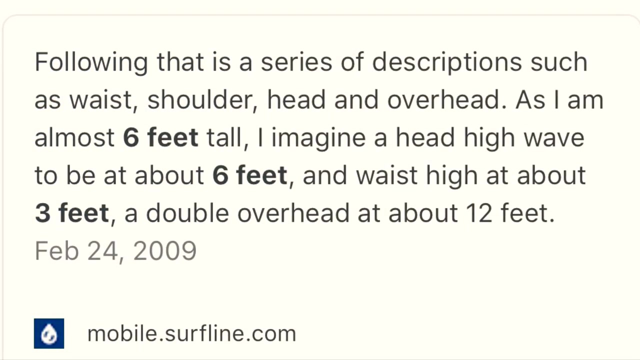 way out, I asked another surfer, pointing to the shore: how big do you estimate the waves out there? puzzled, he said two to three feet. and then I went to surf line, which said this: following that, a series of descriptions such as waist, shoulder, head and overhead: as I am almost six feet tall, I imagine a head high wave to be about six feet and 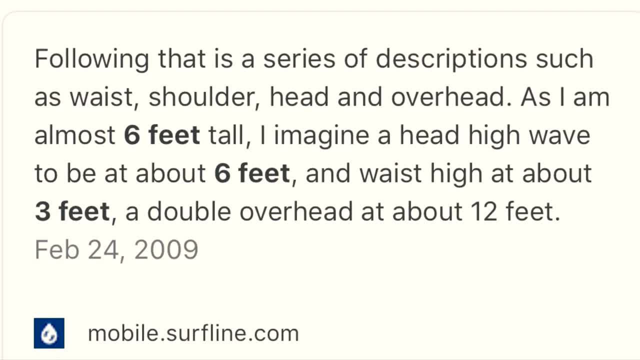 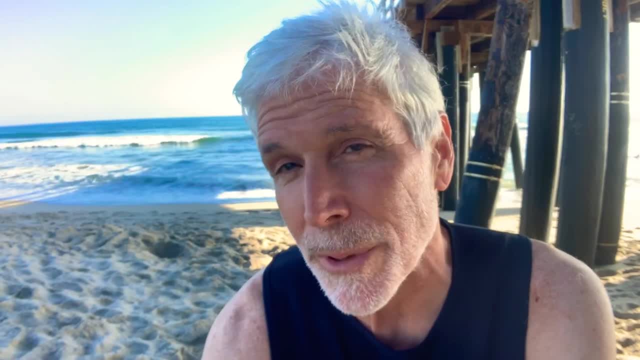 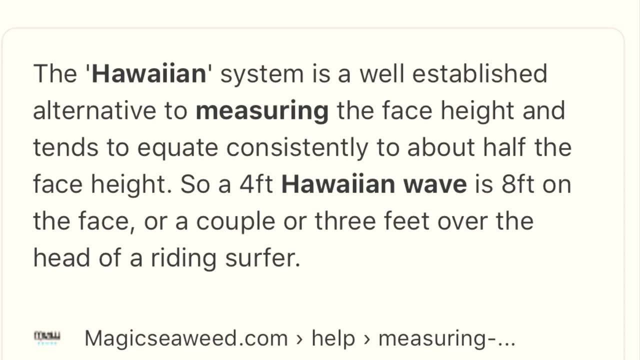 waist high about three feet and double overhead about 12 feet. so I did a little research. I discovered that the surfer dude was trying to beat me in with a little Hawaiian standard of measurement. the Hawaiian system is a well-established alternative to measuring the face height and tends to equate consistently to. 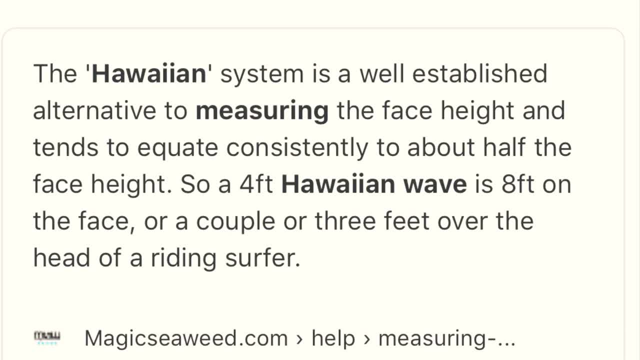 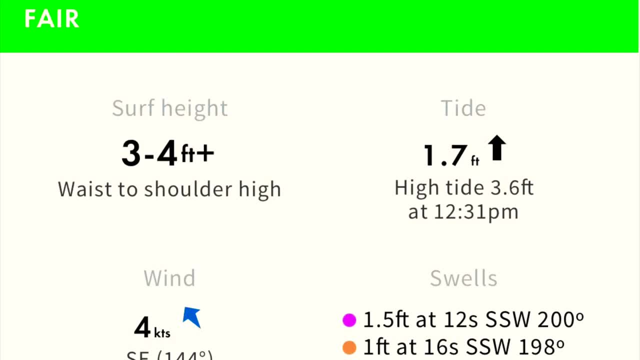 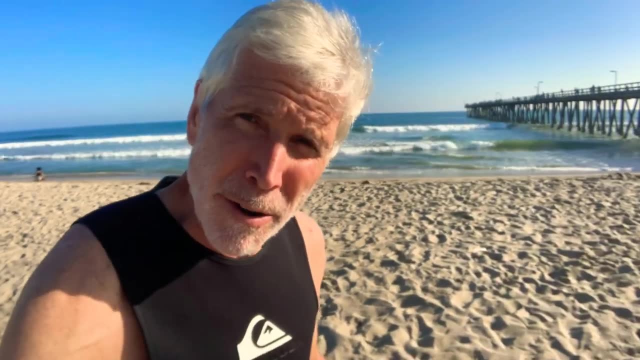 about half the face height. so a four-foot Hawaiian wave is interesting to me. eight foot on the face, or a couple or three feet over the head of a riding surfer. the forecast from surf line for Malibu Lagoon that day was three to four feet, and then, with a little more poking around on the internet, I found this guy. 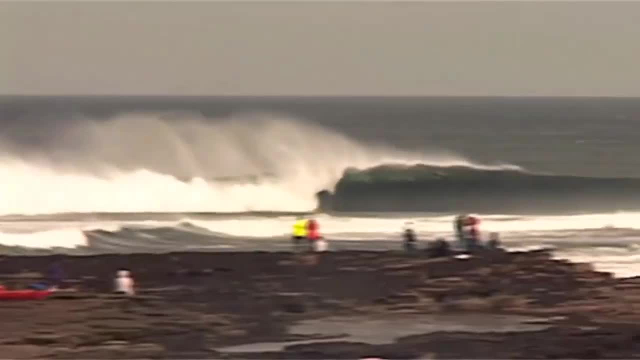 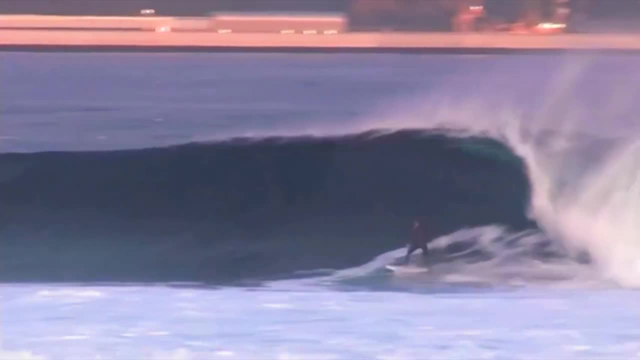 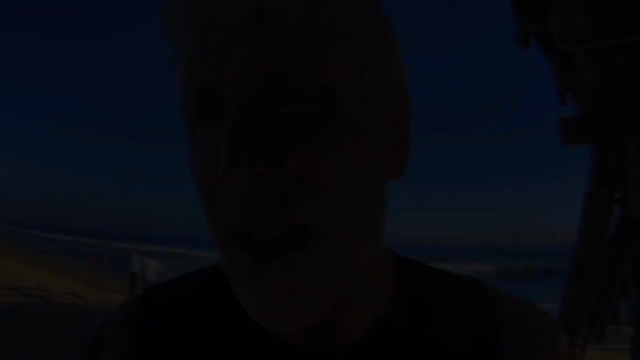 and I think he had a pretty good solution, like the best way to measure waves is to just say it's head high, it's double overhead, its knee high, its ankle barrels, etc. now in my five years at SoCal I've learned that there's some pretty cool.